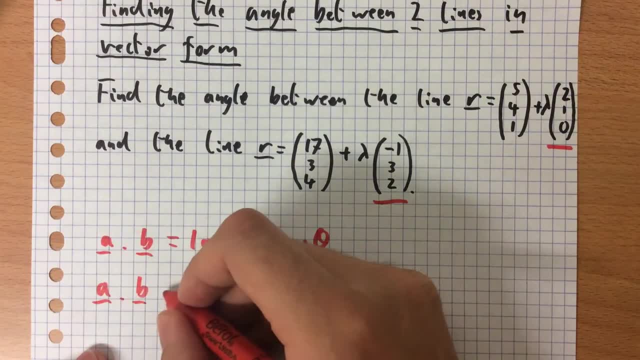 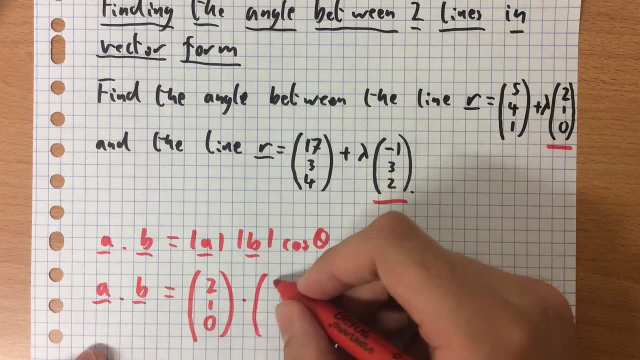 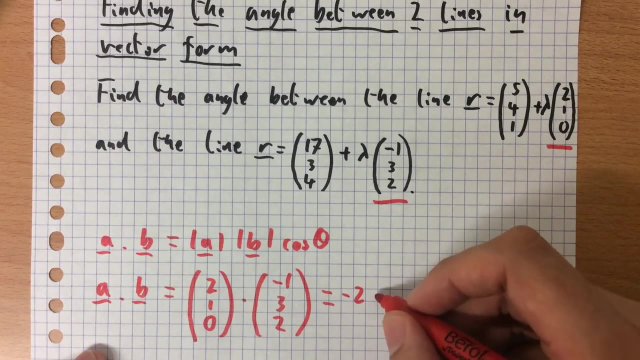 So a dot b is equal to 2, 1, 0.. Dot minus 1,, 3, 2,, which is equal to minus 2, plus 3, plus 0,, which is 1.. Oh, that's a nice easy thing to deal with. 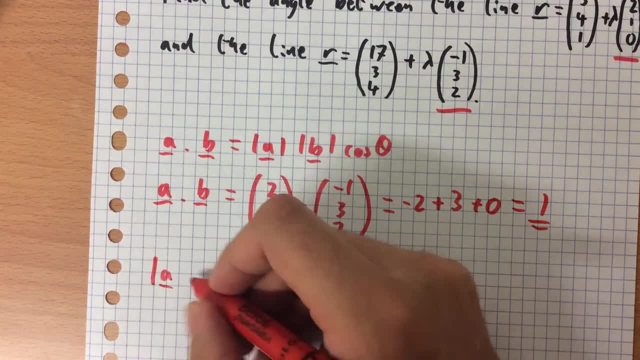 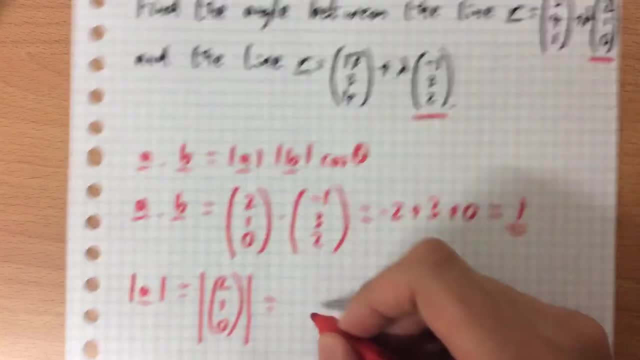 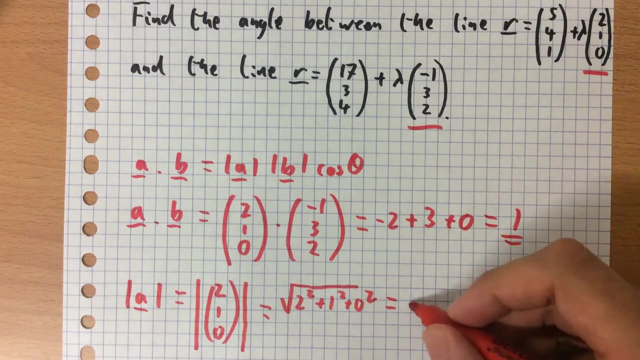 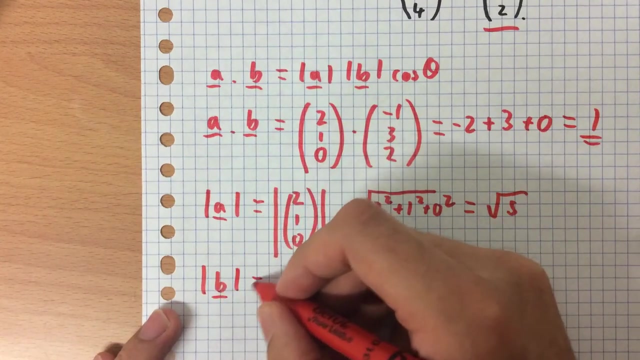 The modulus of a is equal to the modulus of 2, 1, 0.. Which is the square root of 2 squared plus 1 squared plus 0 squared, which is the square root of 5.. And the modulus of b is equal to the modulus of minus 1, 3, 2.. 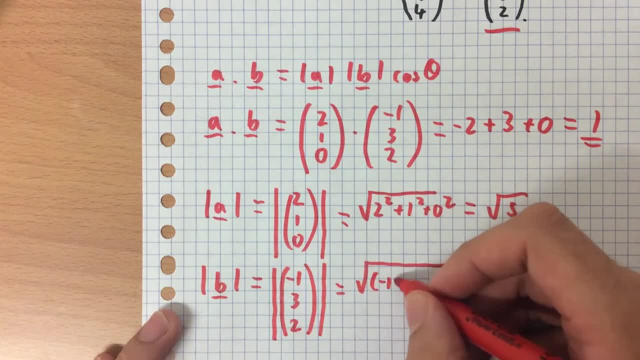 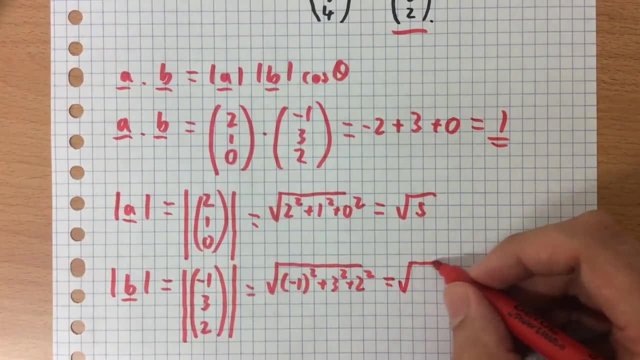 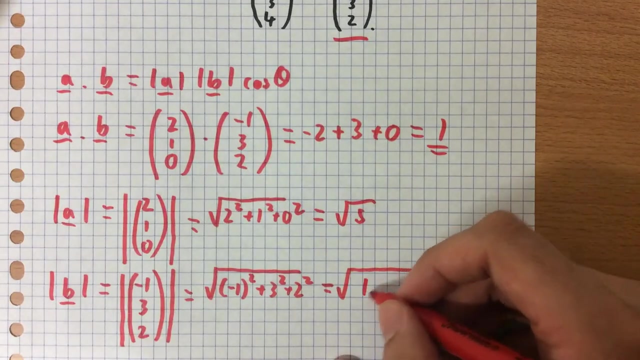 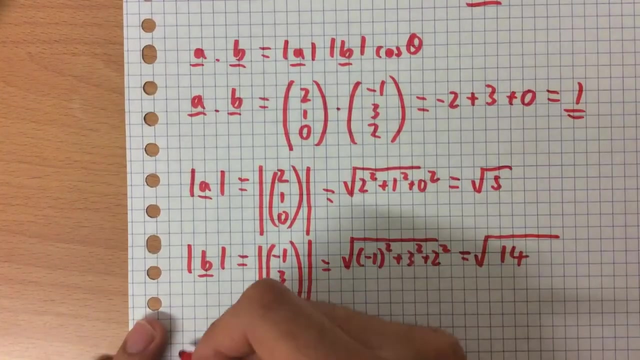 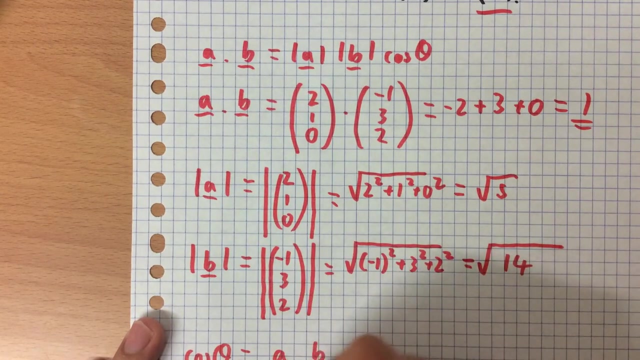 Which is the square root of minus 1 squared plus 3 squared plus 2 squared, Which is, Which is The square root of 1, plus 9, plus 4, square root of 14.. So now we use rearranging this equation to make, cos theta is equal to a dot b all over: mod a, mod b. 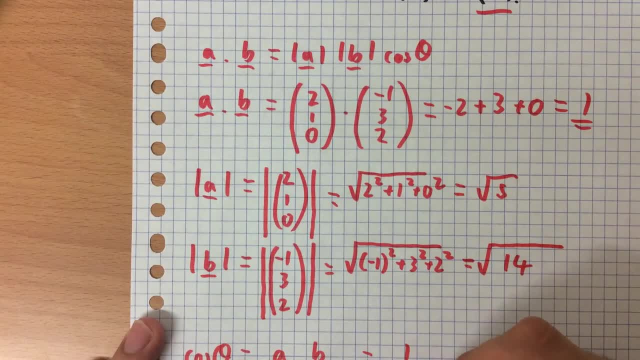 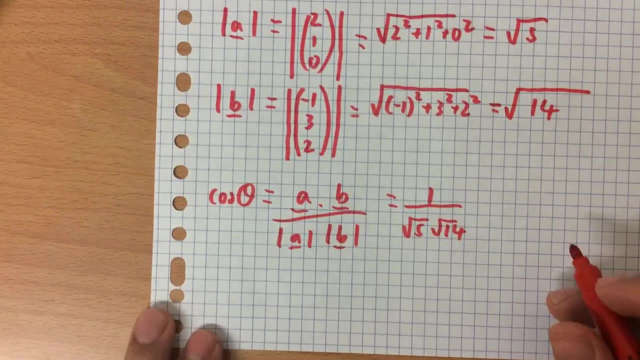 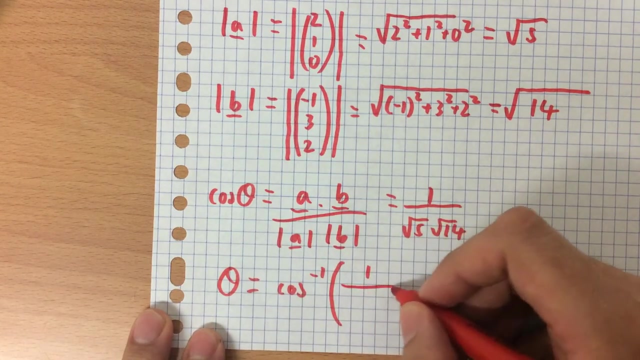 That's 1 over root 5, root 2.. That's 1 over root 5, root 14.. So, lastly, theta is equal to cos to the minus 1 of 1 over root 5, root 14.. 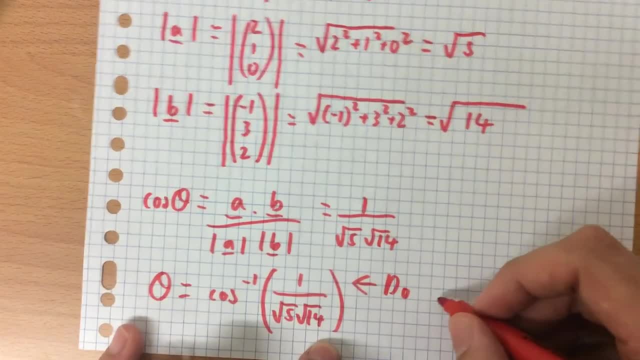 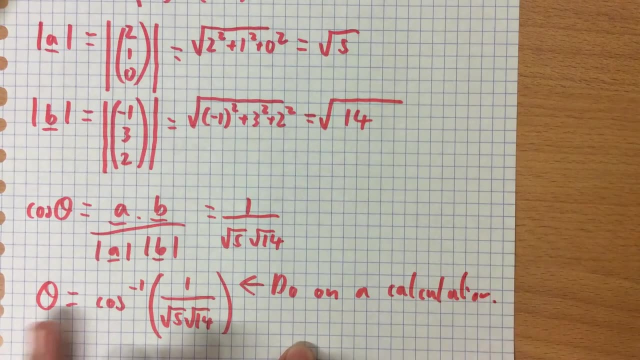 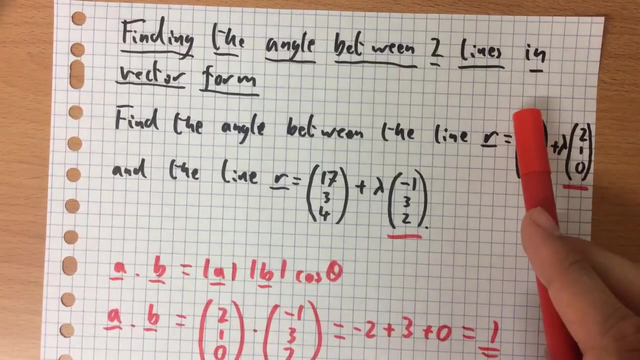 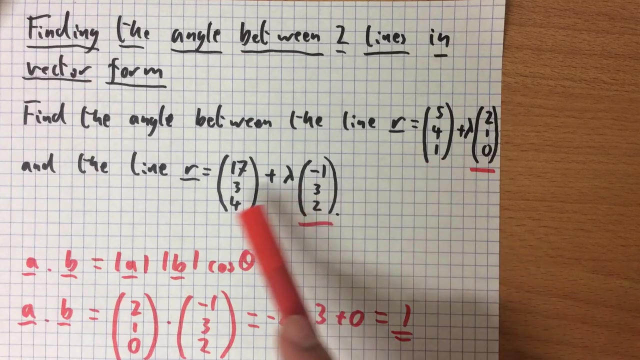 Which you do on a calculator, Easy as pie, Okie dokie. So that is how to find the angle between two lines. The key point is just the same as two vectors. You just use the directions. You completely ignore the bits, the constant vector, part of the line equations.